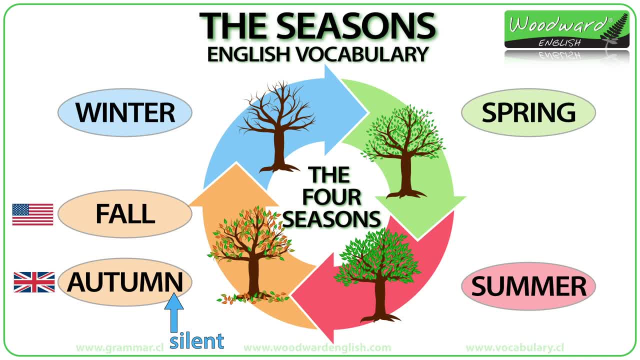 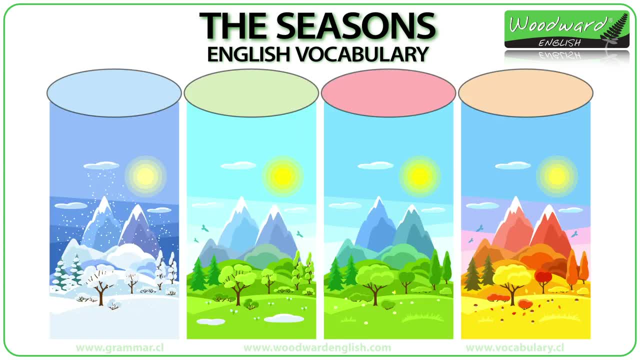 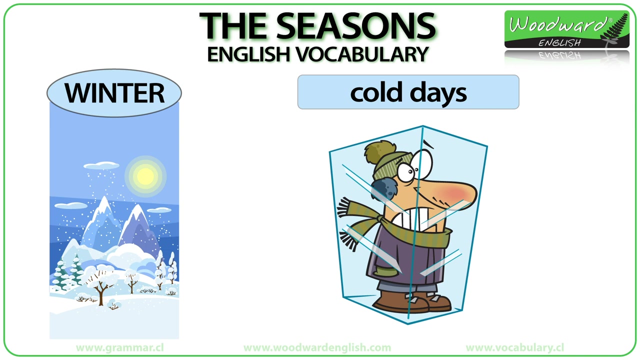 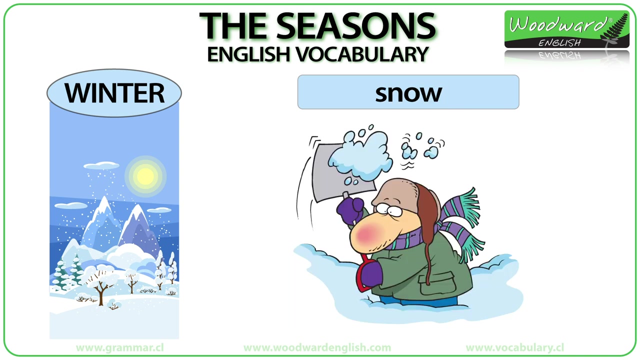 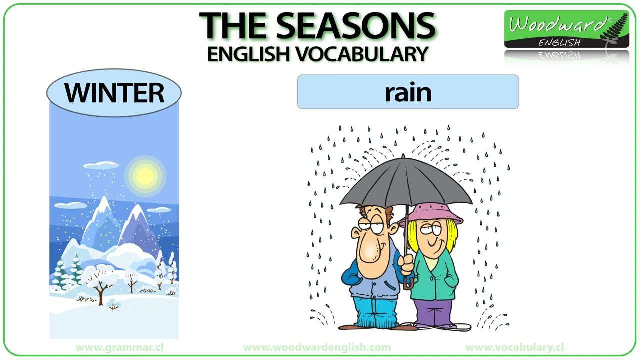 It is silent. autumn, autumn. What are the names of the seasons in English again, winter, spring, summer, autumn. Sometimes autumn is called fall. Let's look at some typical English vocabulary associated with each season: winter vocabulary, cold days, cold days, snow, snow, rain, rain, umbrella. 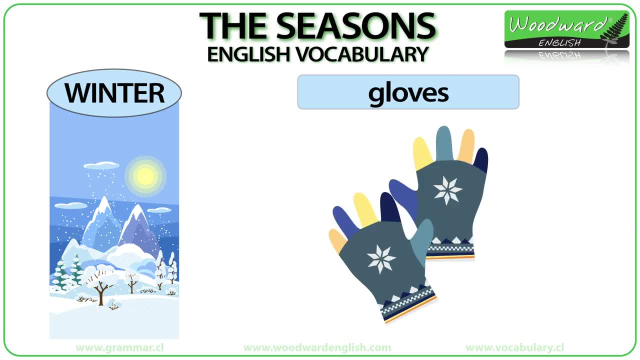 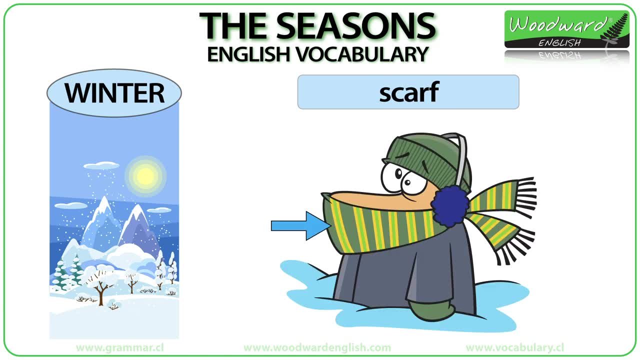 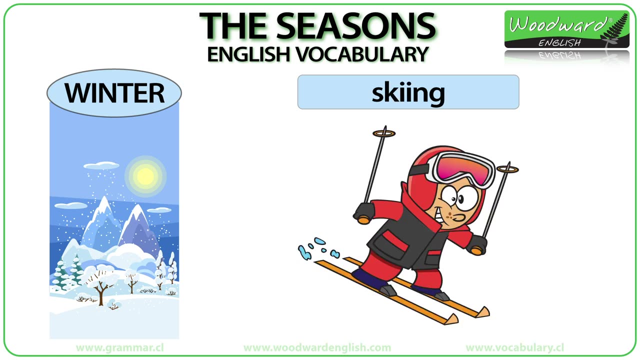 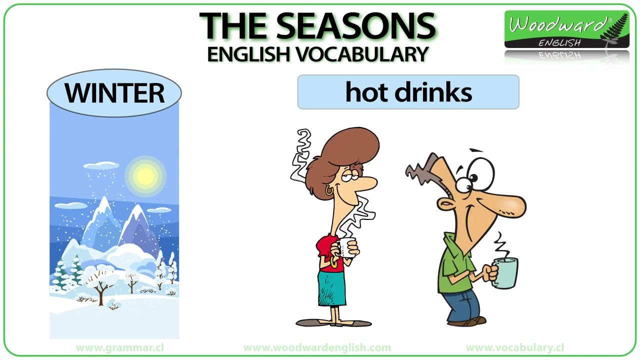 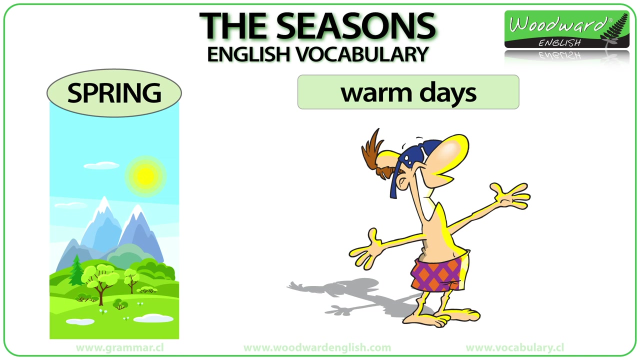 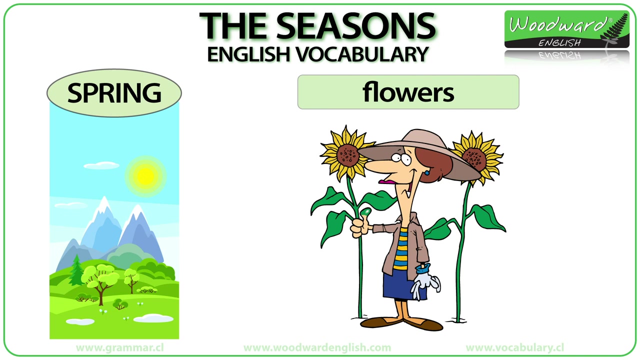 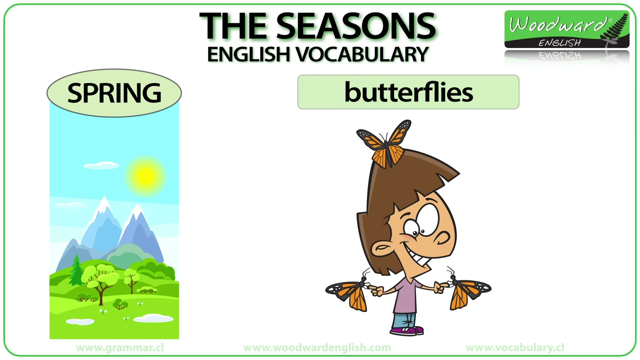 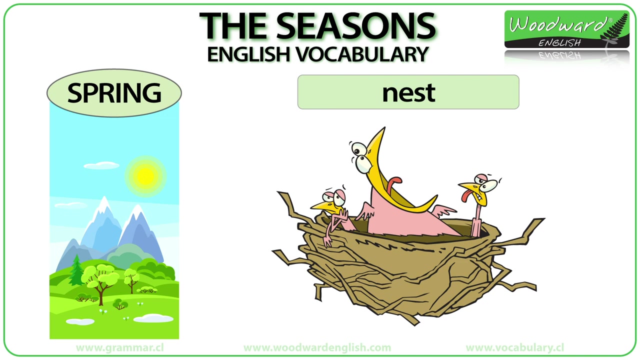 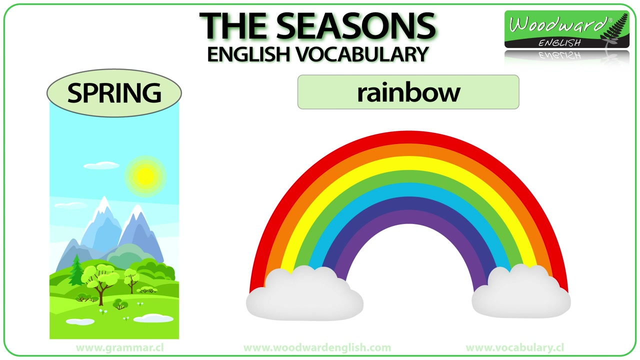 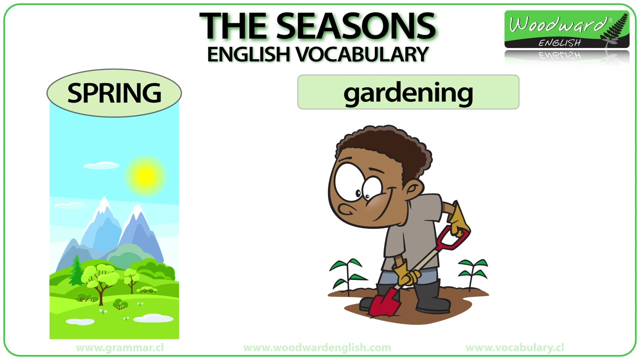 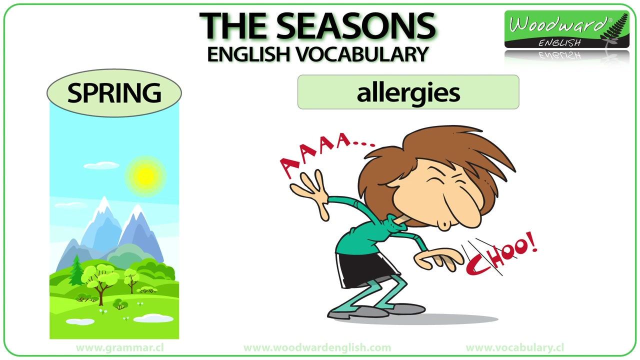 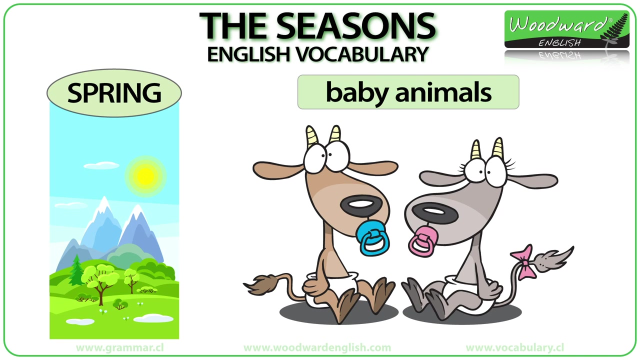 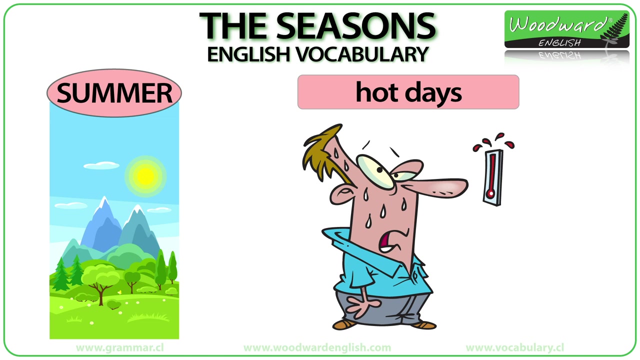 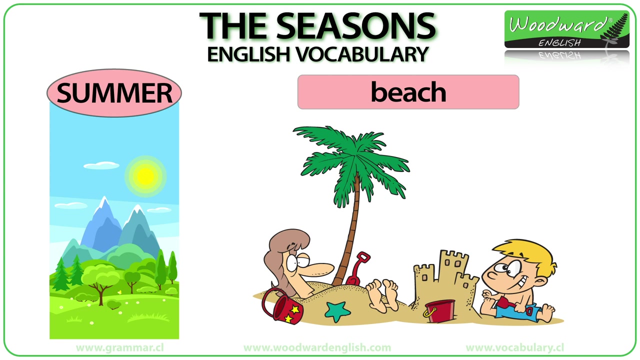 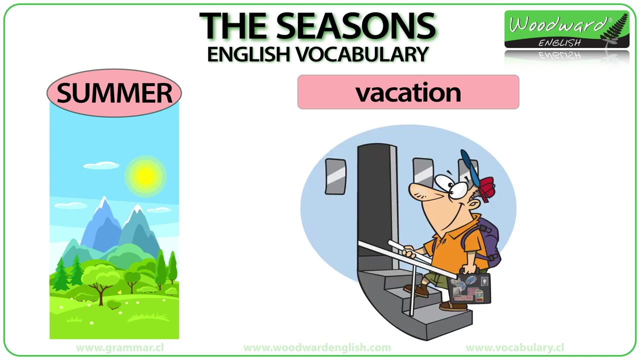 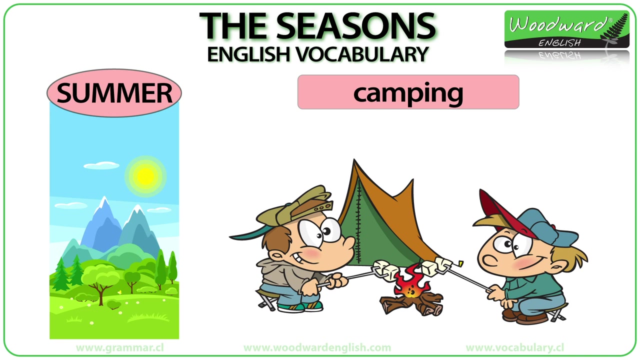 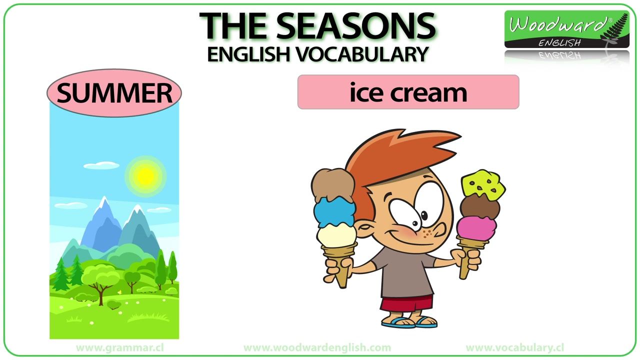 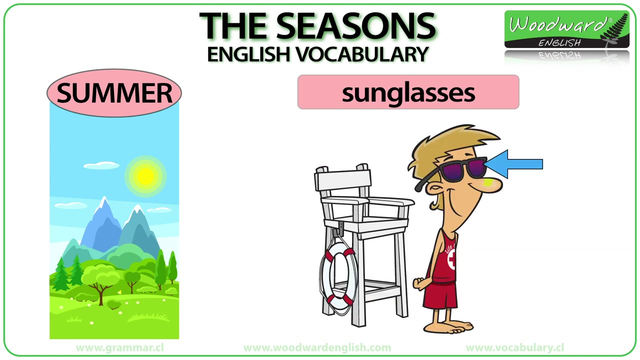 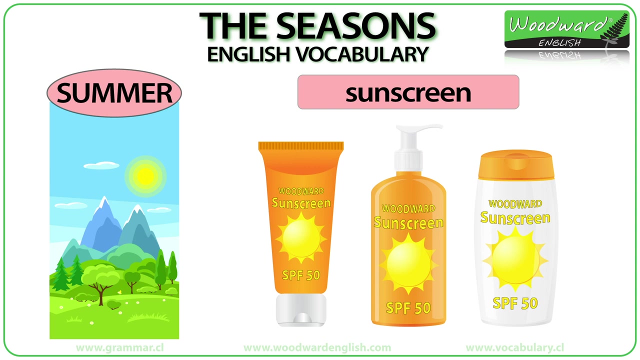 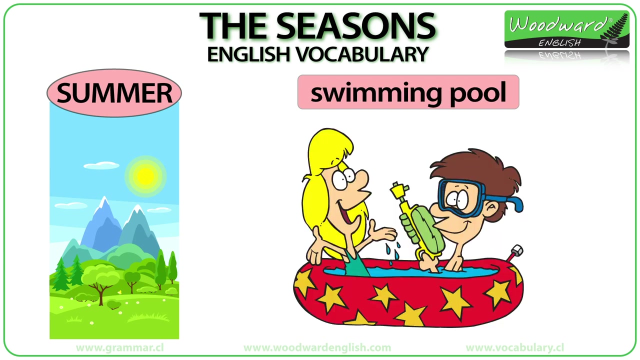 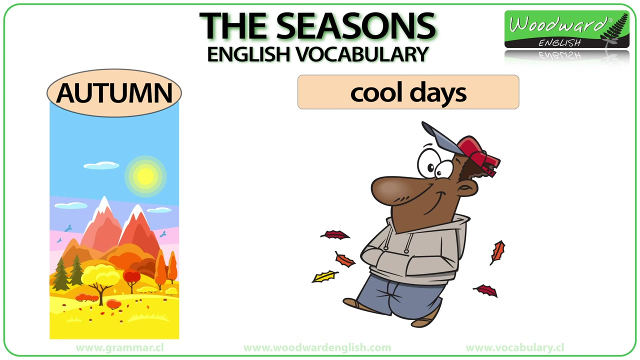 umbrella, gloves, gloves, scarf, scarf, skiing, skiing, hot drinks, hot drinks. spring vocabulary, warm days, warm days, flowers, flowers, butterflies, butterflies, butterflies, butterflies, nest, nest, rainbow, rainbow, gardening, gardening, allergies, baby animals. summer vocabulary, hot days, beach vacation, camping, ice cream, sunglasses, sunglasses, sunglasses, sunscreen, sunscreen, swimming pool, swimming pool. autumn vocabulary or fall vocabulary. 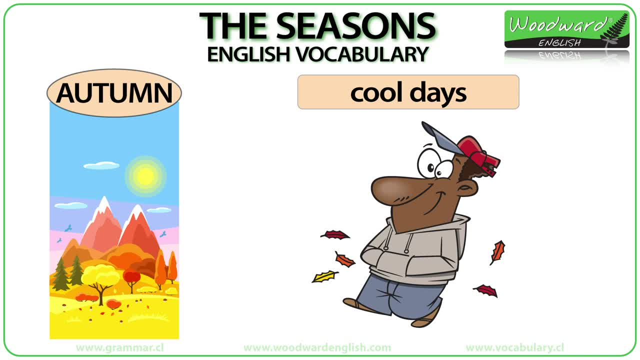 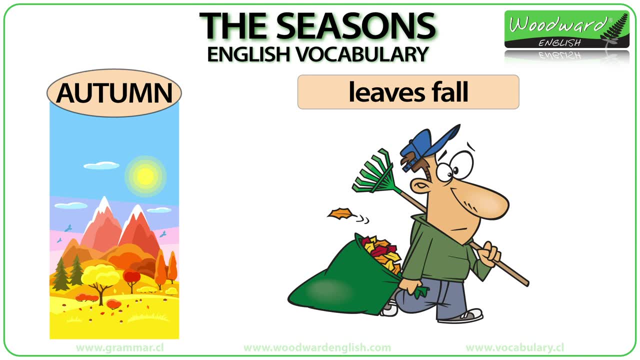 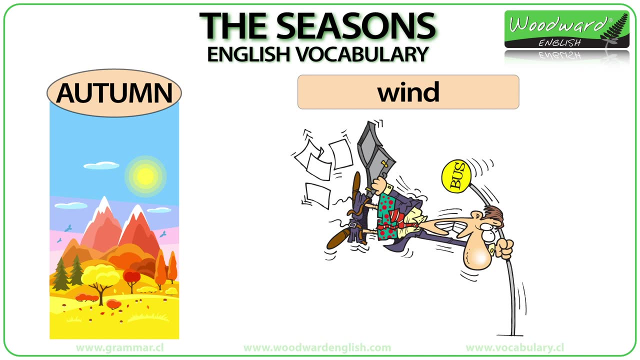 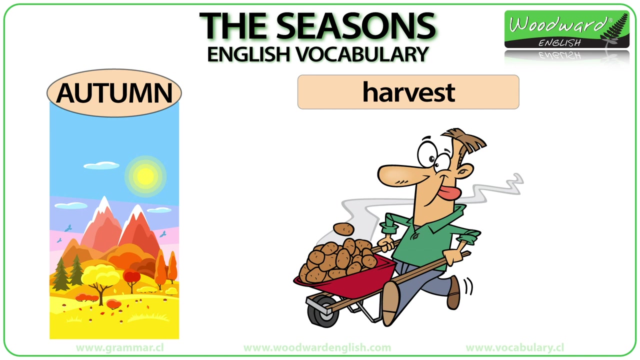 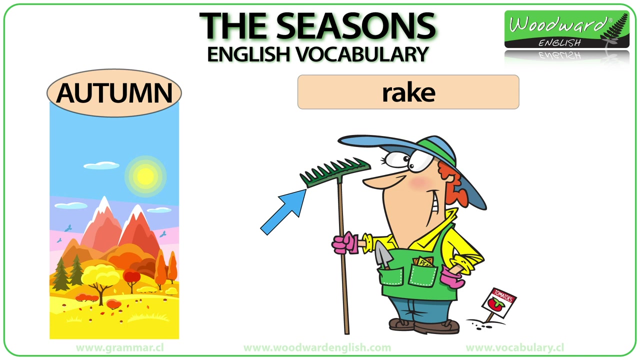 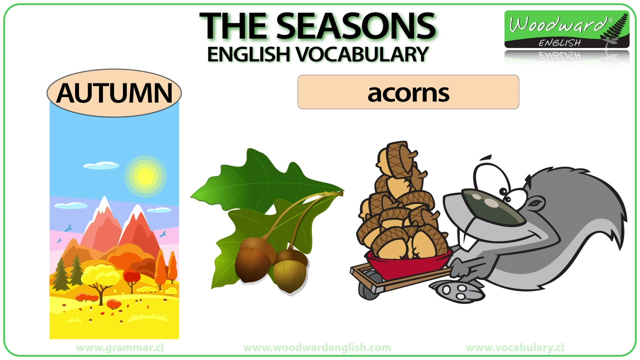 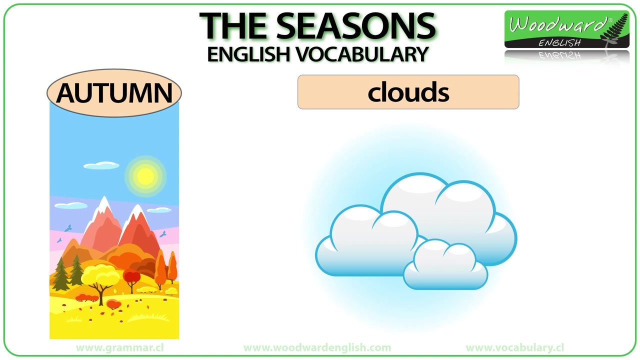 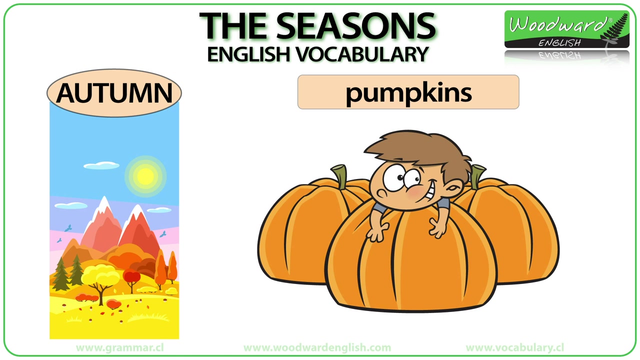 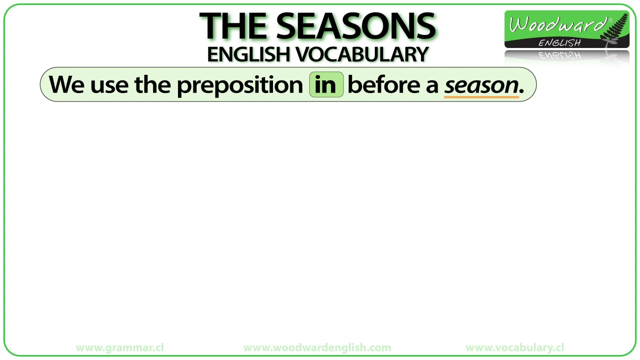 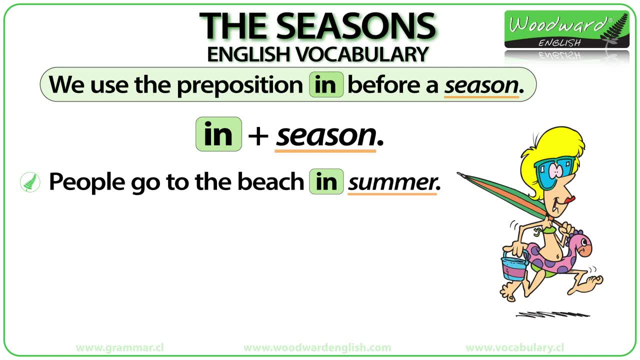 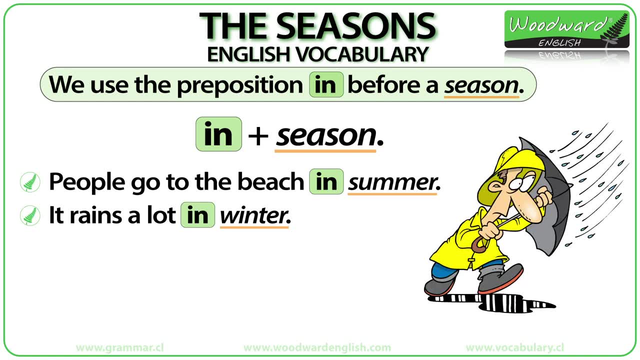 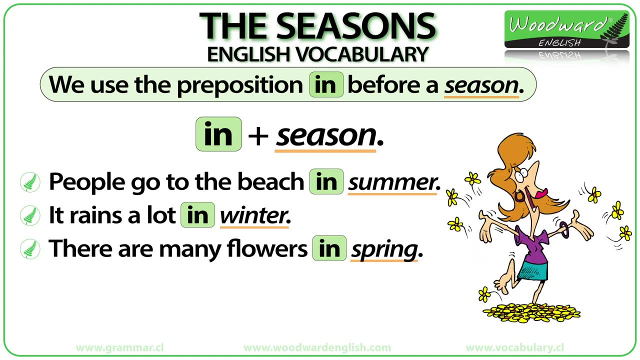 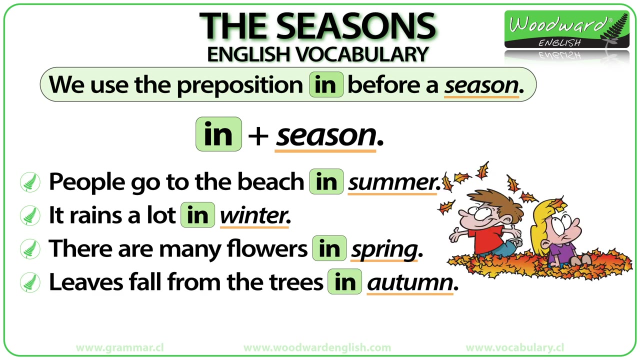 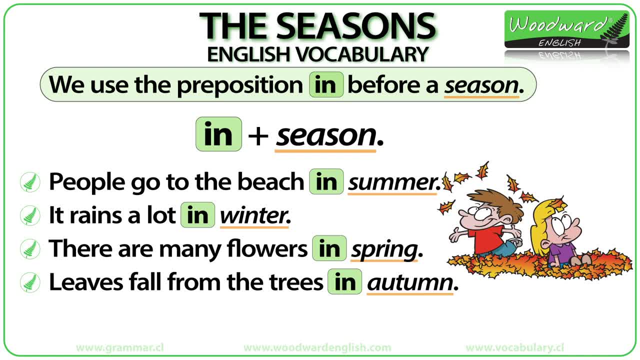 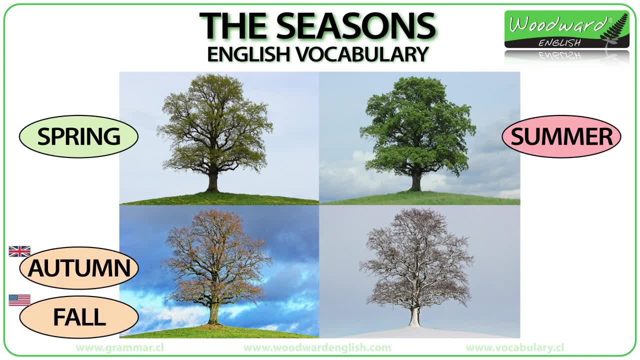 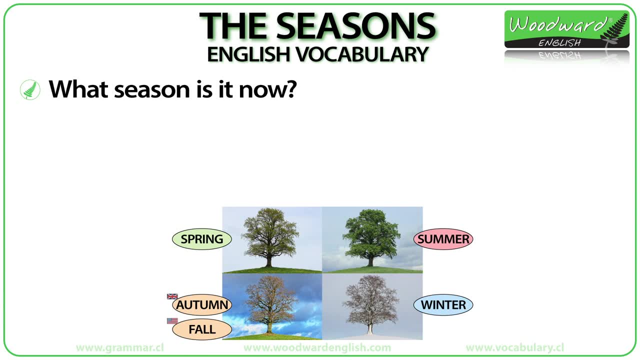 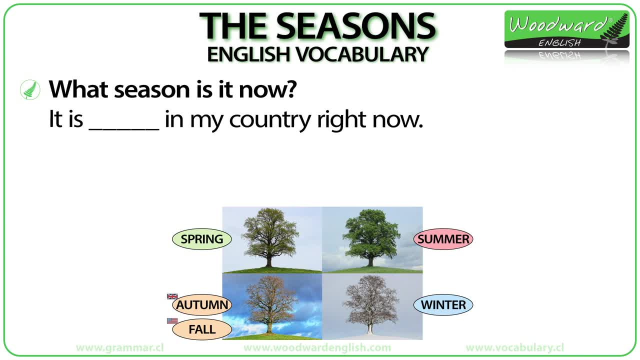